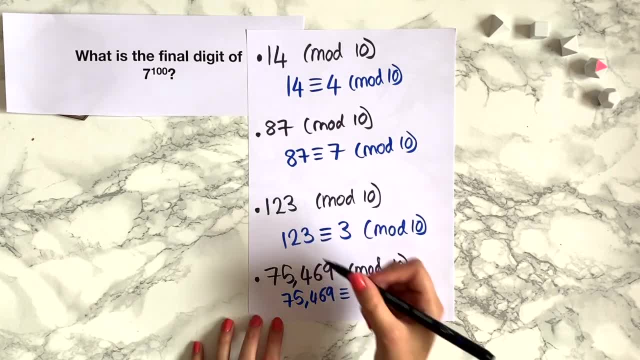 And this kind of makes sense, because if you imagine every number has a zero at the end instead of its actual final digit, that number would be divisible by 10, so that number would appear at the 10 o'clock marker at the top of the clock. Then to get to the 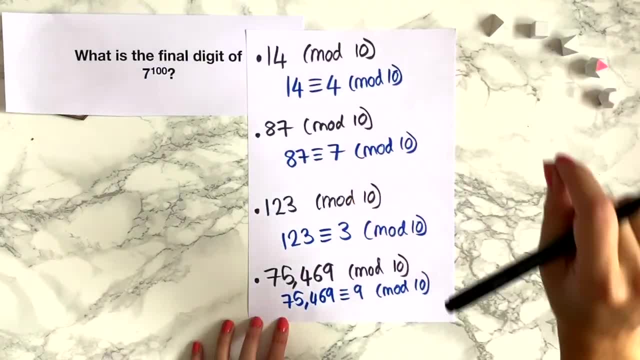 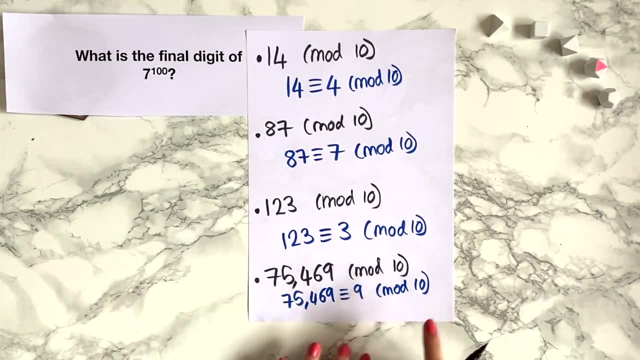 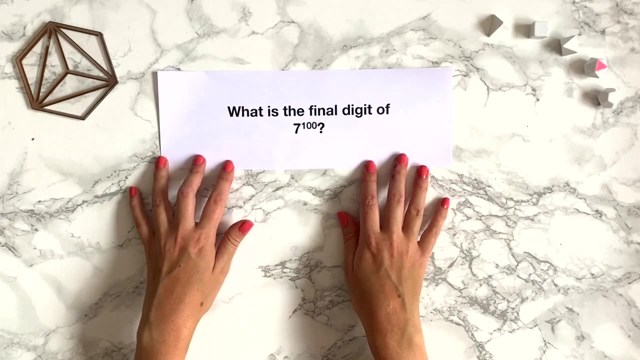 actual number we have to add on that digit and we'd count round that many hours on our clock so we would end up at that number o'clock. So any number taken modulo 10 will produce the final digit of that number. So this is really interesting for our question here. 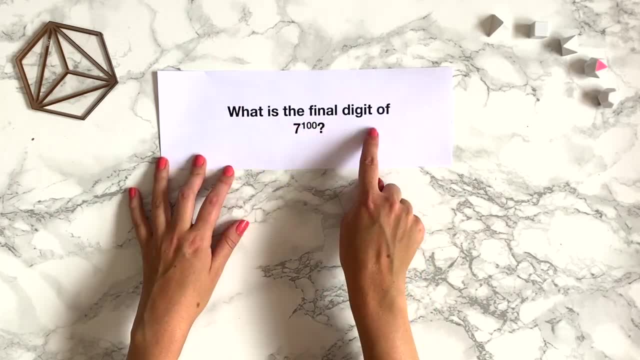 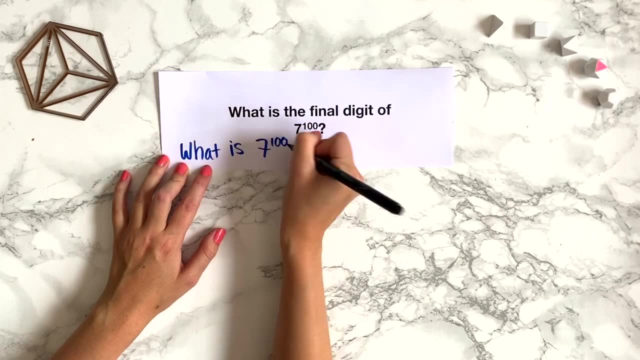 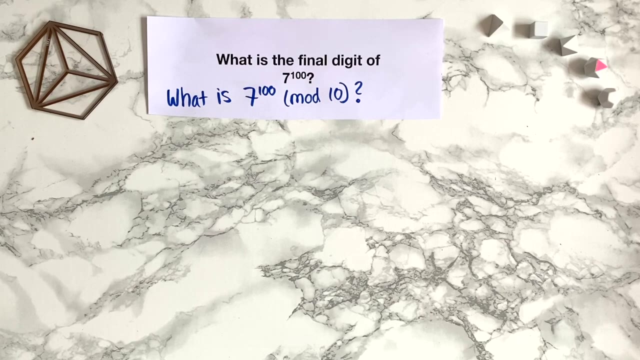 Because it means that this question- what's the final digit of seven to the power of a hundred- is actually the same as asking what is seven to the power of a hundred modulo 10.. And so suddenly this question is a lot more approachable if we use modular arithmetic. Now let's have a think about: 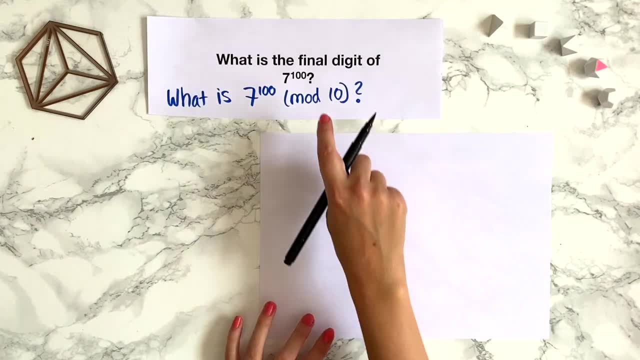 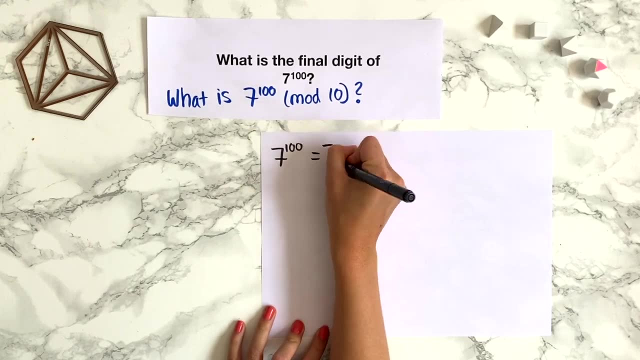 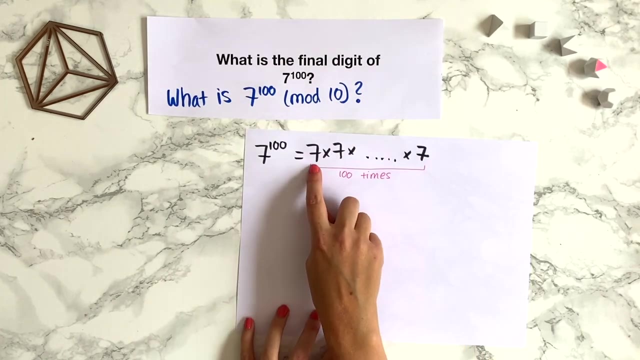 how we can solve this question. So a really good first step, when you have big powers and you're doing a modular arithmetic style question, is to remember that seven to the power of a hundred is just 7 times 7 times 7, 100 times. So now we're trying to evaluate this big product: modulo 10. 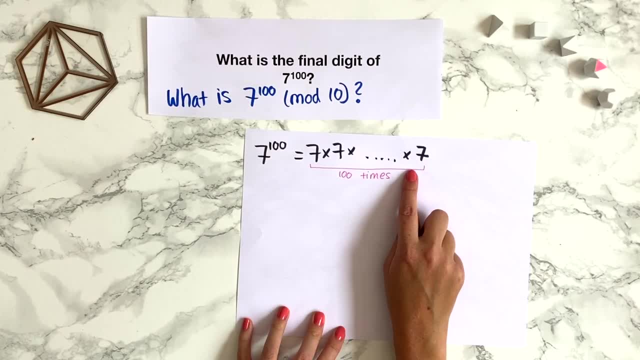 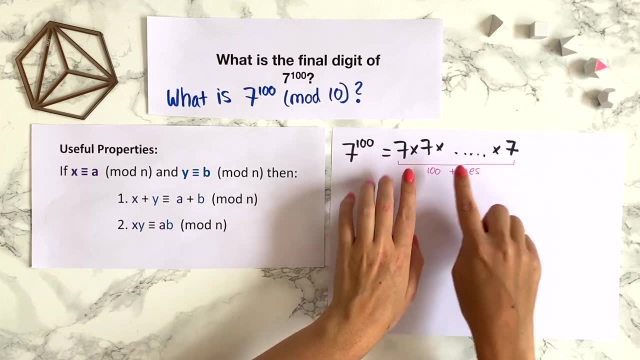 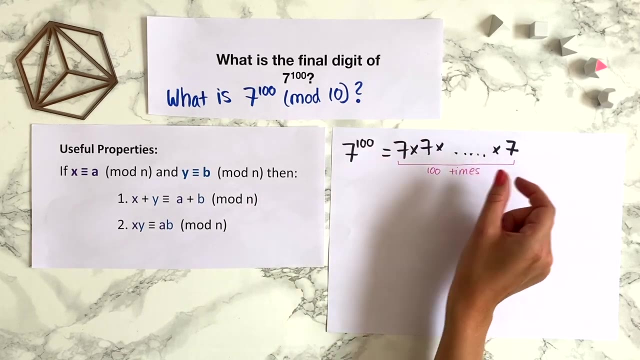 and because we have a product, we would quite like to use our theorem about products in modular arithmetic. So remember, our theorem says that instead of working out 7 times, 7 times, 7, 100 times, and then taking it modulo 10, instead we can work out individual components of the 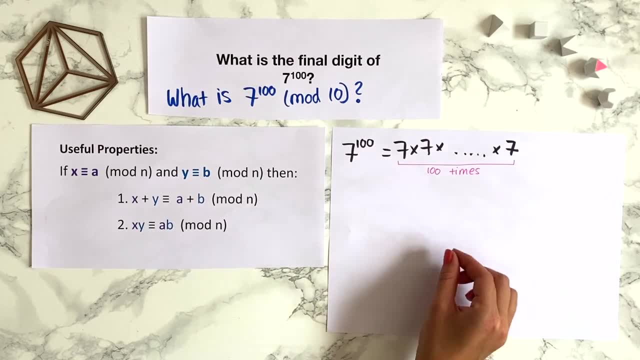 multiplication modulo 10 and then multiply the result of that together. But hold on a moment, because 7 modulo 10 is just 7.. 7 is already as reduced as possible in mod 10.. So this theorem currently isn't looking too helpful. However, what we can do is group the 7s in this multiplication. 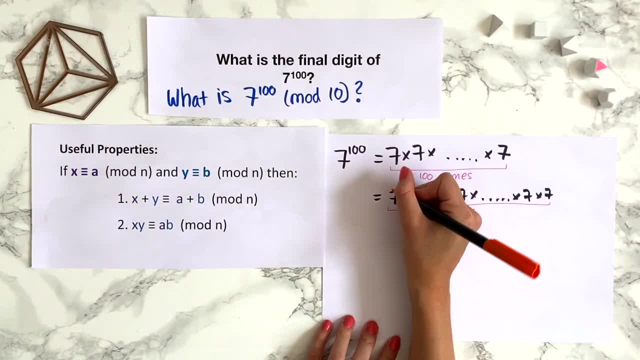 Let's say we pair up the 100 7s, So we're going to multiply these two 7s together and these two 7s together. and then we're going to multiply these two 7s together and these two 7s together. 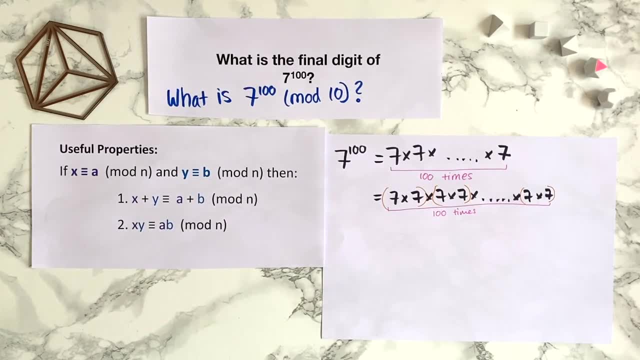 And then so on, and then until we get to the final pair. So there are 50 pairs of 7 times 7s. 7 times 7 is 49. So we can write this as 49 times 49, and so on 50 times. 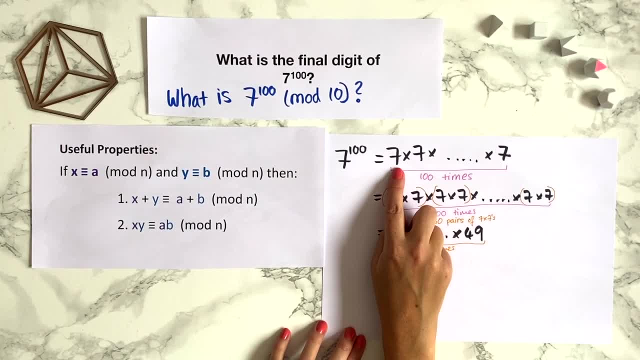 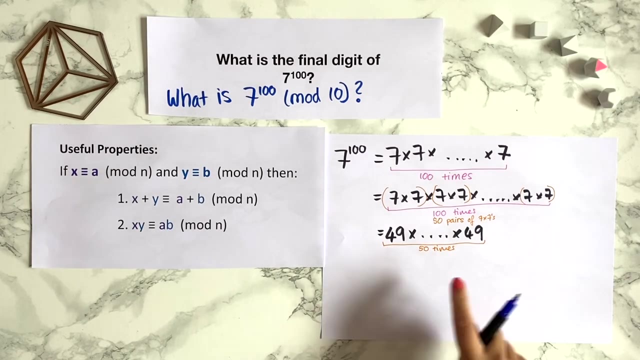 So we couldn't reduce the 7s modulo 10 before, because 7 was already reduced as much as possible. So this theorem didn't really help us. But now we've got 49s So we can use this theorem because we can reduce 49 modulo 10.. Let me write this on the side So: 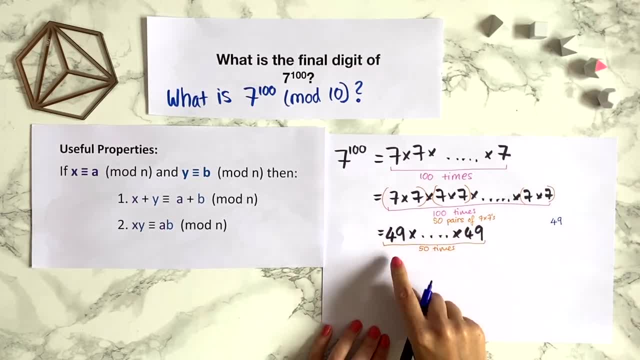 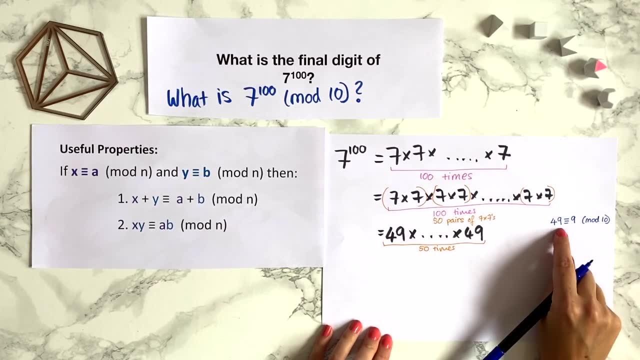 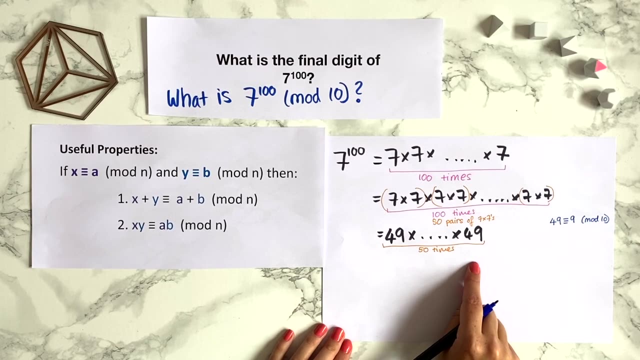 49,. well, modulo 10, 49 is congruent to 9.. Remember, mod 10 really just takes the final digit of a number, So we could rewrite this as 9 times 9 times 9, and so on 50 times. But that's still quite a hard. 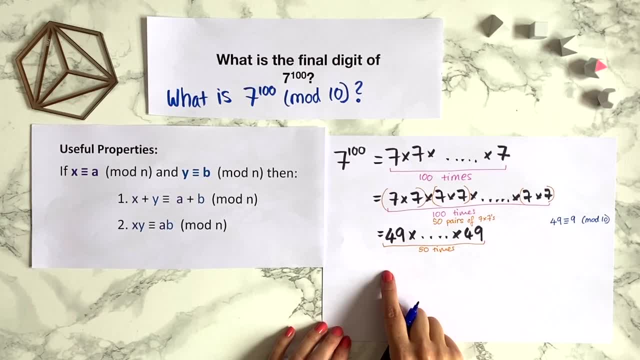 product to work out. We don't really want to calculate the number of times 9 times 9.. So we're going to take 9 times 9 times 9 and then work out what that is modulo 10, because that's quite hard. 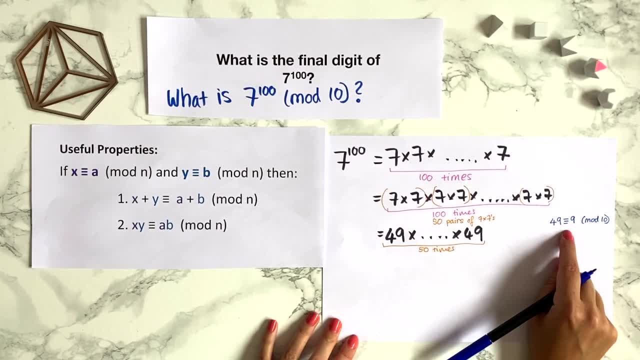 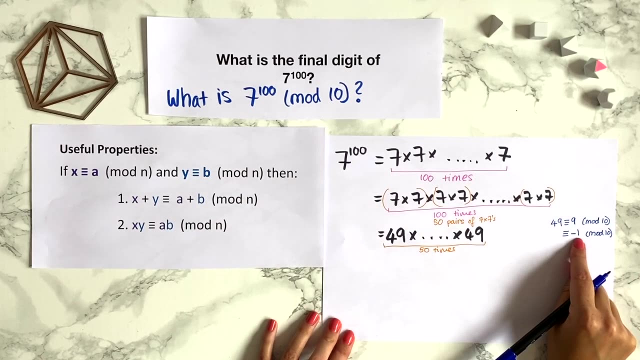 to compute. But actually, is 49 congruent to anything else that's helpful? Well, 49 is also congruent to minus 1 modulo 10.. Perhaps the easiest way to see that is to think about the spiral representation we covered in the intro video. If you continue coiling the number line round into 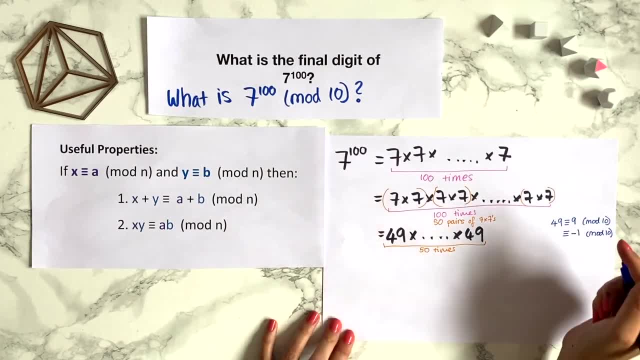 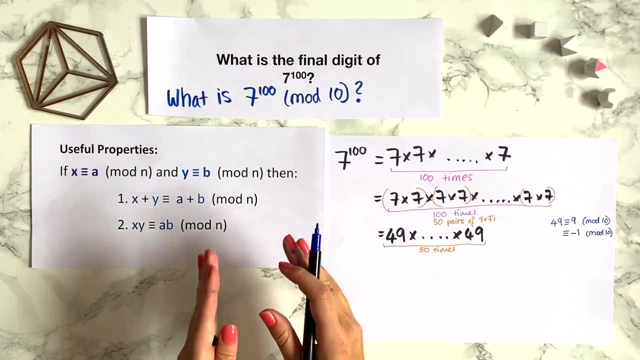 the negative section, minus 1, would appear underneath the 9.. Alternatively, you could also subtract 10 from 9, you get minus 1.. And so say you're at 9, if you add 10 and add 10 and add 10 or 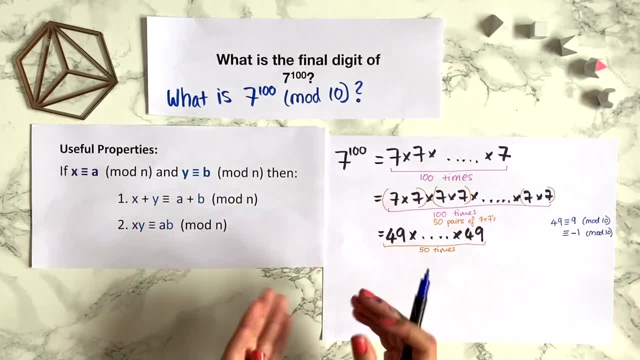 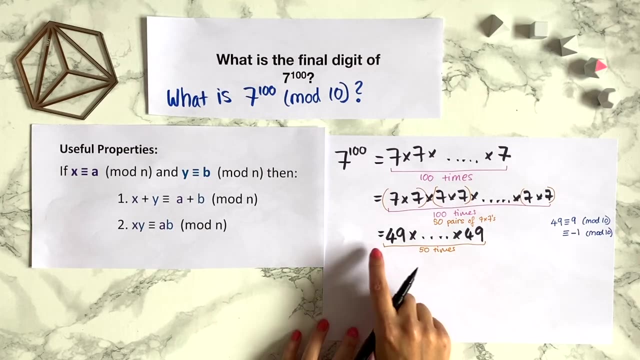 subtract 10 and so on, you'll keep hitting numbers that are also congruent to each other. So 9 is congruent to minus 1.. So this is really good, because products involving 1, minus 1 or 0 are really good things to aim for, because we can multiply them really easily. So this is actually. 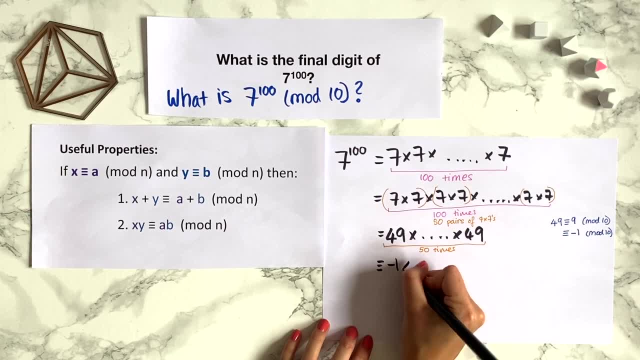 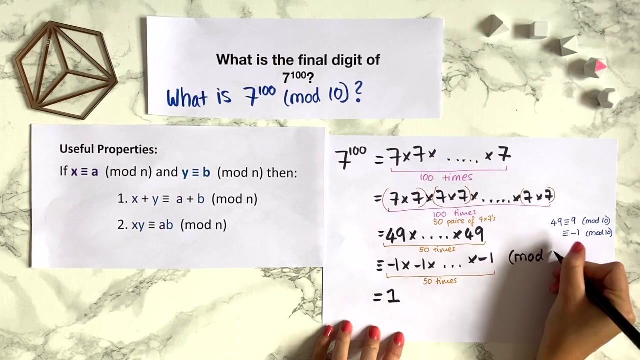 congruent to minus 1.. Here's an example of a question for you guys. It asks this question: What is So? that's our answer. 7 to the power of 100 modulo 10 is 1.. And this means that the final 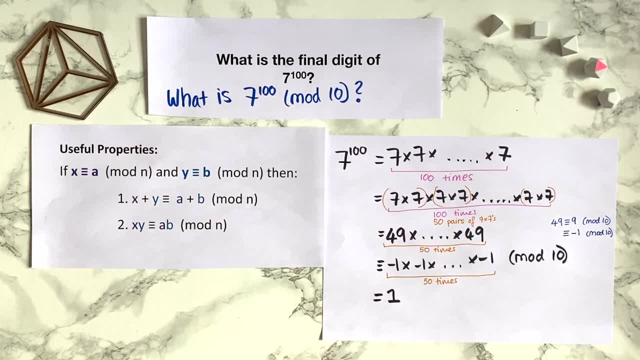 digit of 7 to the power of 100 is only the register of all of those digits. So now let'space a function like a 1. 7 to the power of 100 is 1.. So there we go. we've once again made quite an intimidating question.